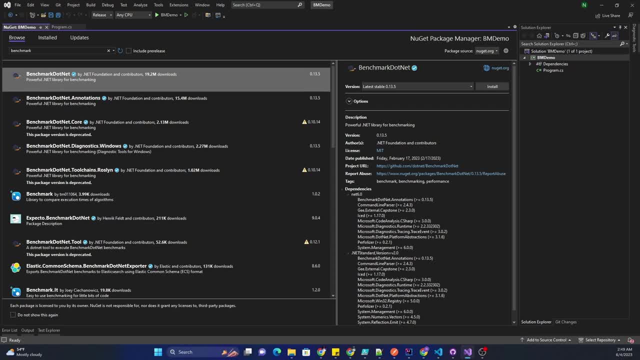 performance measurement. It also allows us to measure the impact of different optimizations and tracks the improvement over time, which is extremely important. It also can compare the performance of multiple code implementations or different algorithms to determine the most efficient solution for a specific scenario. It provides statistical analysis and metrics to support a data-driven decision-making process. 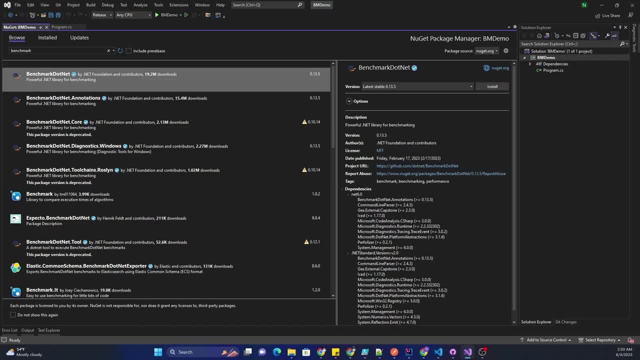 It also facilitates an iterative development process by allowing us to benchmark and measure the performance of our code as we make changes and optimizations. It helps us validate the impact of our changes and make informed decisions during the development lifecycle. So I'm going to go ahead and install this NuGet package. 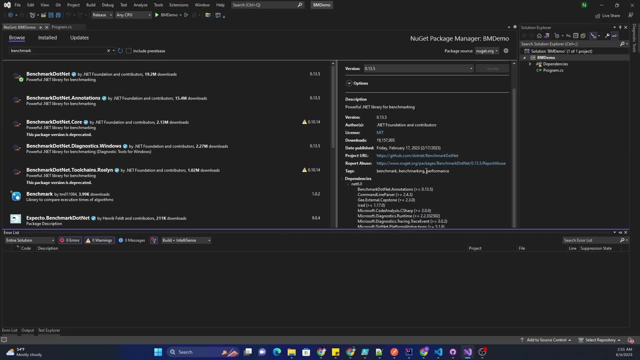 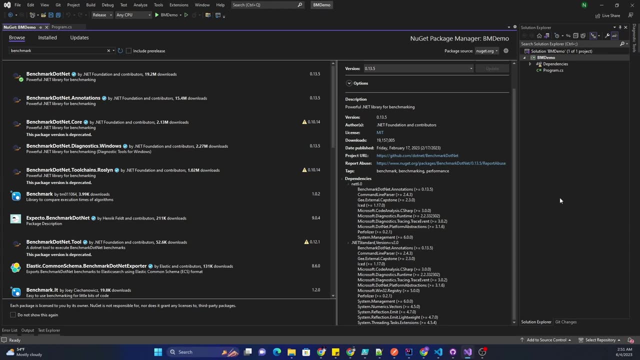 And apart from these advantages, as you can see here, the benchmarknet is the best way to implement dot-net 6 as well as dot-net standard, which means it supports different environment and frameworks for benchmarking, meaning Linux Windows as well as dot-net. 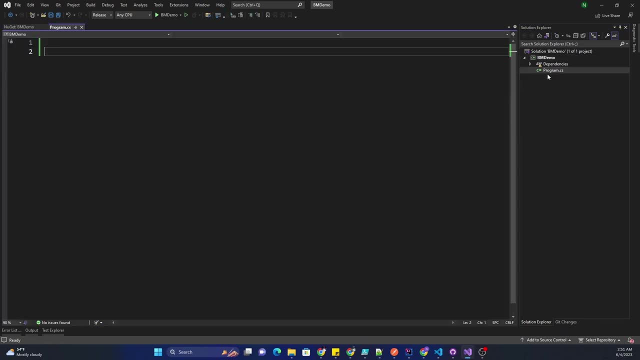 legacy and newer version of dot-nets. So now for the simplicity of the example. I'm going to take a very simple scenario which we are going to benchmark, But in a real-life example. the benchmarking need only occurs for very complex and CPU. 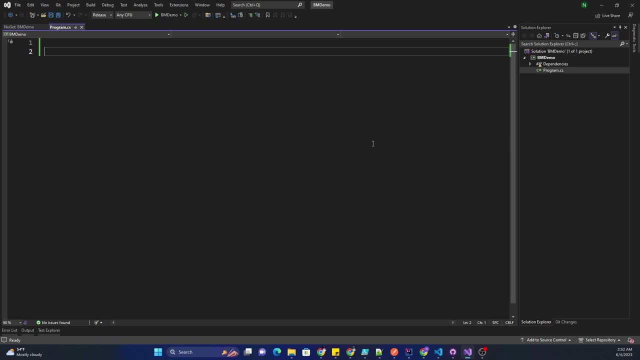 or performance-intensive code which we need to benchmark Again. benchmarking just a HTTP call might not be a very good use case. The reason for that is an HTTP call will behave the same. there is not much to change to improve its performance. 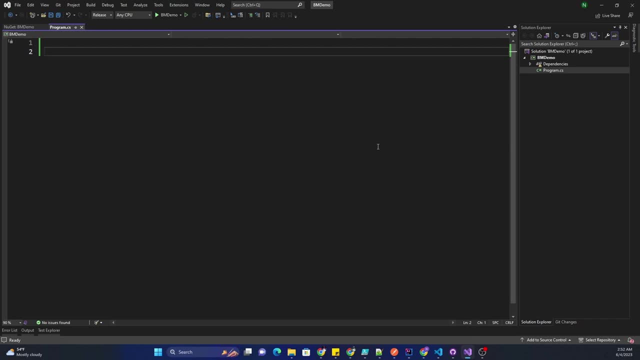 Whereas in a real-life example, the benchmarking need only occurs for very complex and CPU or performance-intensive code, which we need to benchmark. So what we're going to do is, after we get a response from an HTTP request, if we implement. 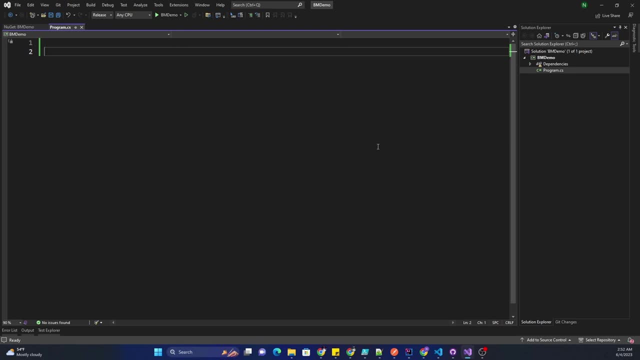 some sort of complex logic to transform the data and apply some algorithm. that part of the code might be a good candidate for benchmarking. Now for the purpose of this application, let me create a simple class. Now, most of the example out there uses things like this. 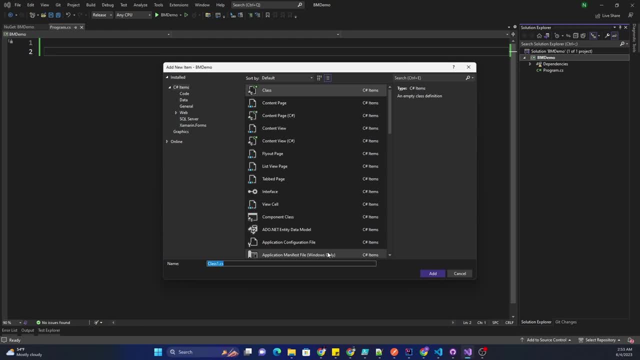 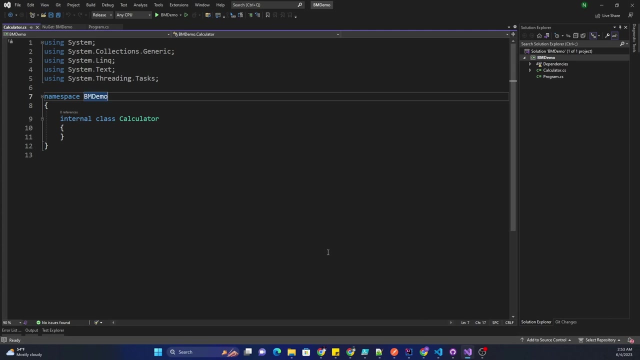 Things like encryption. But for this example, I'm going to use a very simple implementation, Just an implementation of addition, So we can create a calculator class, And one thing to keep in mind is that the class needs to be public. And here 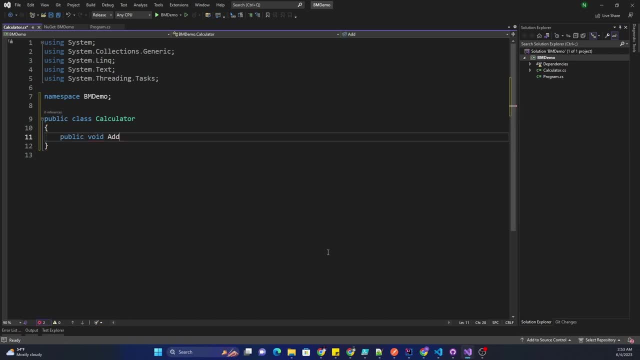 We can create a public void and let's say, we are doing add And we are doing add of two numbers, And this can be just returning first plus second, That's all. So that's all we are going to do. This should be an integer as well. 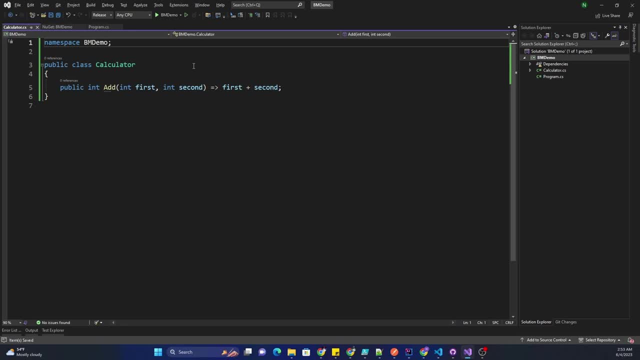 The response type. So that's all we are going to do And this is what we are going to run our performance benchmark on. Again, this is not a very useful use case, but it is going to demonstrate how we can use the benchmark Nuget package. 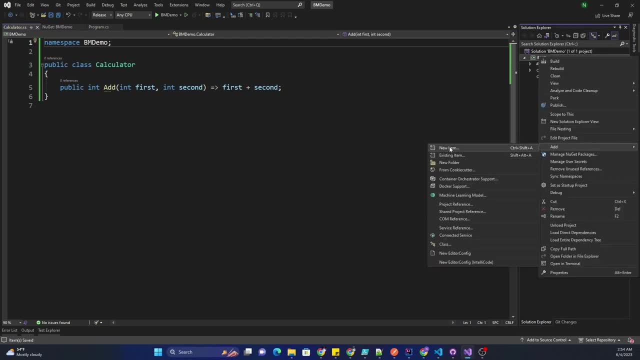 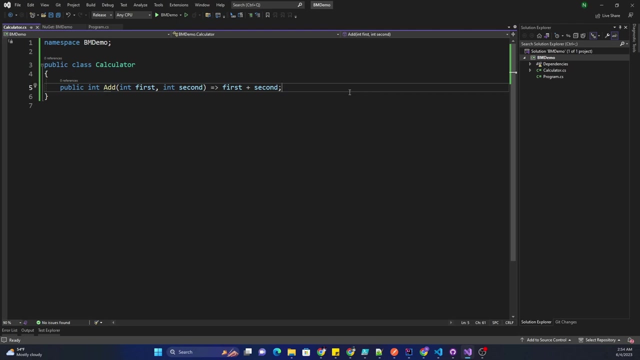 Next, what I'm going to do is I'm going to create a runner which will be responsible for running this code When we use benchmarknet. consider it just like using a unit test. So here, this is the original code, And then we will write some sort of test code for testing the benchmark. 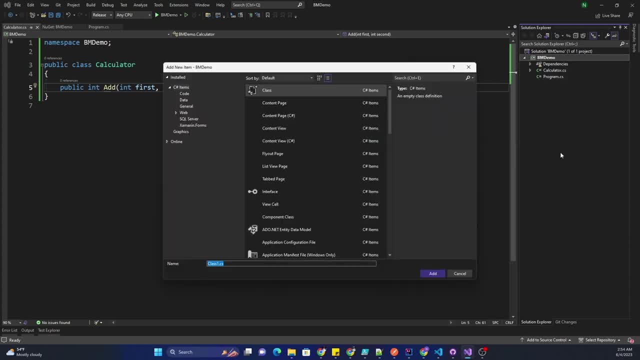 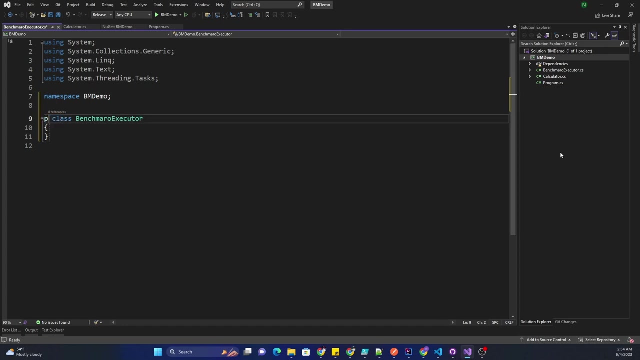 So for that I can go ahead and create a new class And we can say it as a benchmark executor. let's say Similarly this class: also, we need to create it as public And then here- So public void, execute. And what we are going to do here is, inside of this method we can. we can create bar. 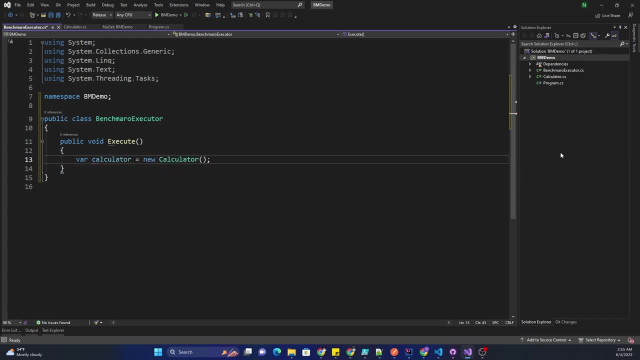 Calculator is equal to new calculator. And then we can do calculator dot add. You can just pass two random number. And here what we can do is we can use an attribute called benchmark, Which is the attribute which will be used by the benchmarking framework to identify. 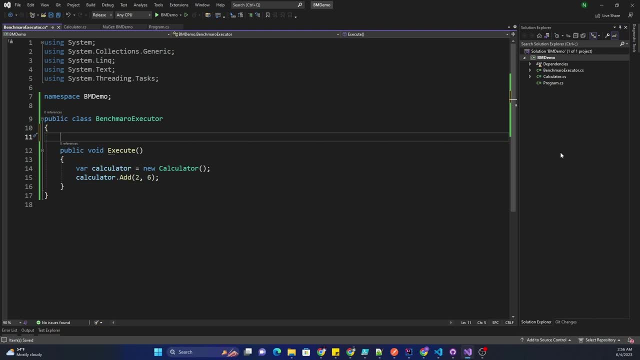 which all method inside a class to be executed for benchmarking purposes. So here I'm going to use benchmarknet- And, as you can see, the benchmark is part of the benchmarknetattributes namespace. And once this is done, I'm going to go into the main method. 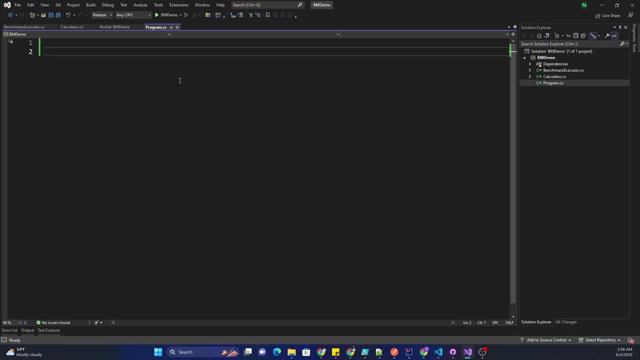 And here what I'm going to do is I'm going to just use benchmark runner. that's the class which is used for running a benchmark nutrii dot run and the run method. we can either pass benchmark running for as you. 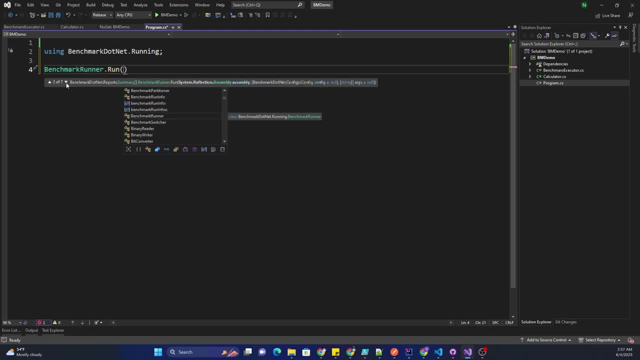 can see on an era of feed or an assembly in which we want to run benchmark or a particular type, with method info on an era of type, And then finally, using fr 같습니다, And then finally benchmark config. but in our case, what we are going to do is we are going to use 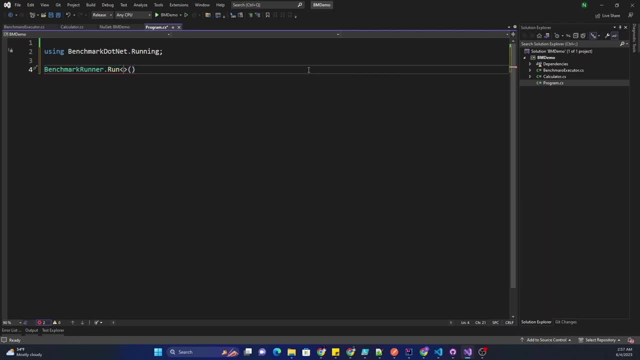 the generic run method and for the generic modern method. apparently I named it as benchmark executor instead of benchmark, so let me just fix this name also and just change it back, and that's all we need to do. we just need to run using the benchmark runner and we need to call the class which will ultimately 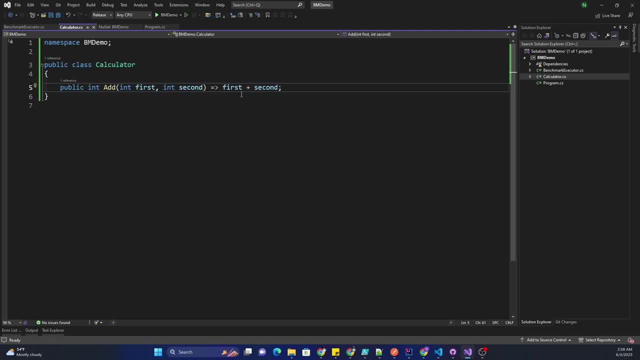 calling the class which is our candidate for benchmark. now, one thing to keep in mind also is that a benchmark cannot be run on a method which takes parameters, because the execution happens at this level. it is going to keep an eye on this. so whoever is calling or whoever is the candidate of benchmark, is like a 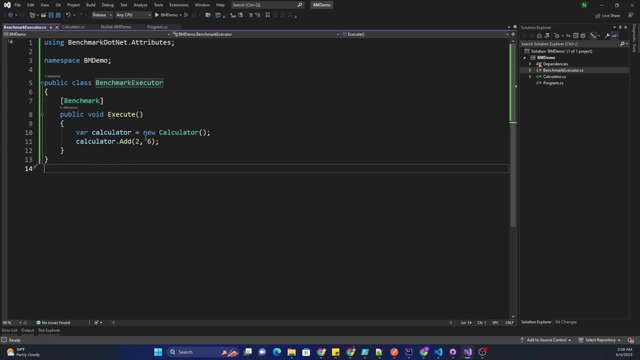 controller which will execute the code that is our candidate for benchmark. so that is something also to keep in mind. so another thing to keep in mind is that if we are running the benchmark, best way to run it is using the release mode, so you can run the benchmark on a method which is running, on a method which is 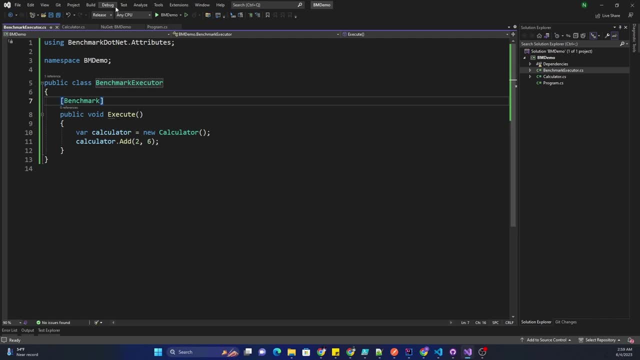 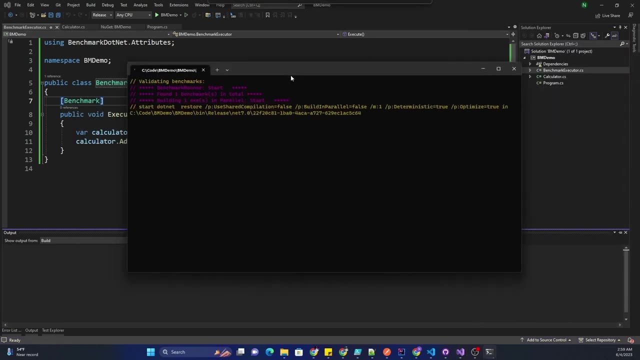 here, as you can see, I'm using release mode. I can go ahead and start without debugging, which is going to open up the command prompt, and in command prompt we can see the benchmark runner has started. it has found one benchmark which it is going to go ahead and run and give us the result. 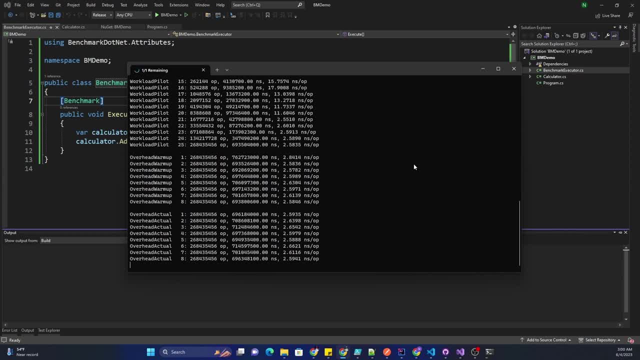 and it is executing bunch of scenarios and finally it is going to present us with the final result, which is what we would be looking into, and here I'm just having one method, but in a real-life scenario we would have at least couple of methods which will be. 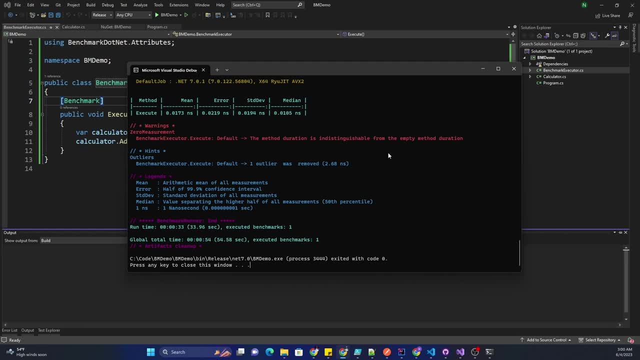 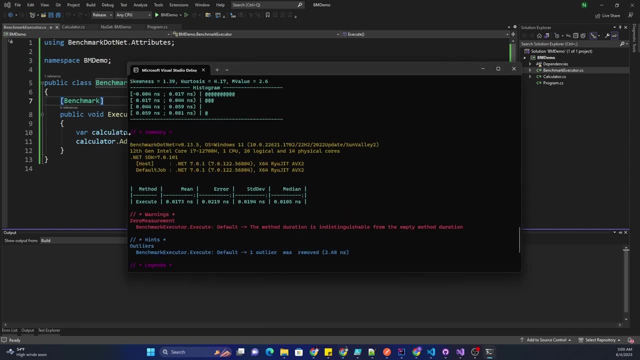 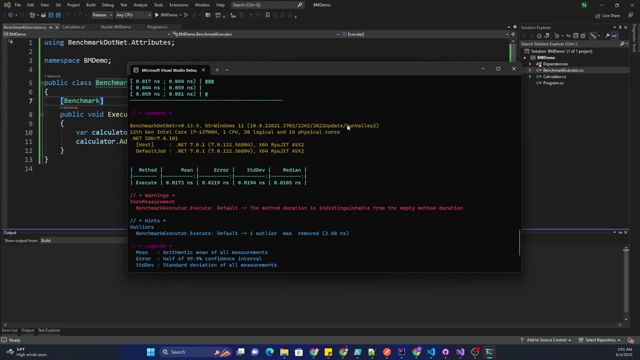 used for comparing between two different implementation. so here this is the final output, and in the output we can look into just the summary tab and this shows which portion of benchmark dotnet it is using, what operating system we are running, in which CPU that it's been used and the version. 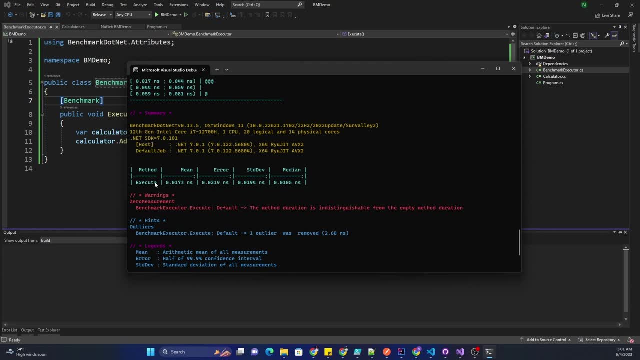 of dotnet. and then it is showing the method, which is execute method. it is showing the mean that represents the average time taken by each iteration of of the benchmark method. and then here it's a standard deviation, and this indicates the standard deviation of the measured times representing the variability of the result. 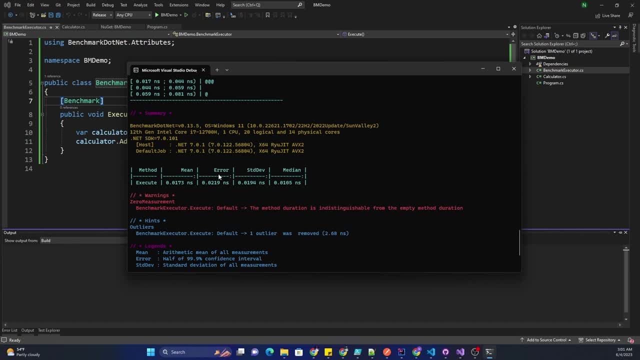 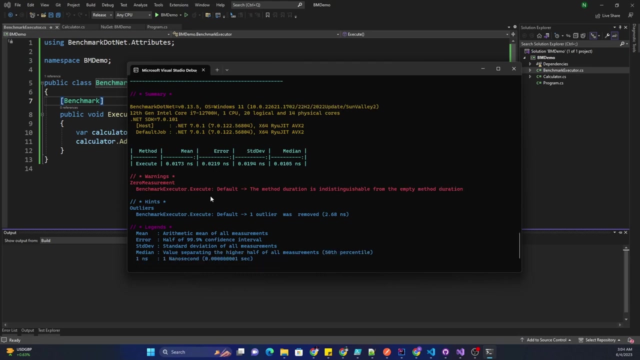 and finally, here the error in this case means standard error of the mean. it represents the standard deviation of the sample means and provide an indication of the precision or variability of the benchmark result. and then, finally, this is the maiden value and looking into this, we would be able to understand how our algorithm is performing. so this gives a very high level.